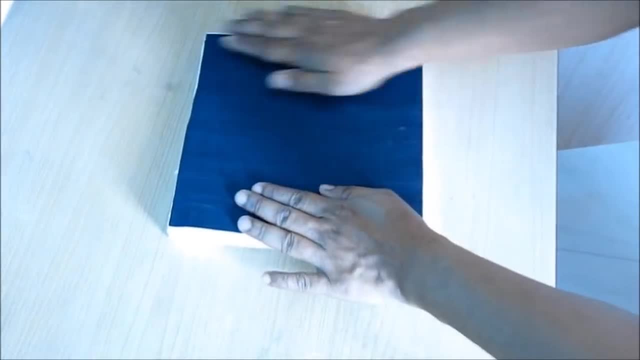 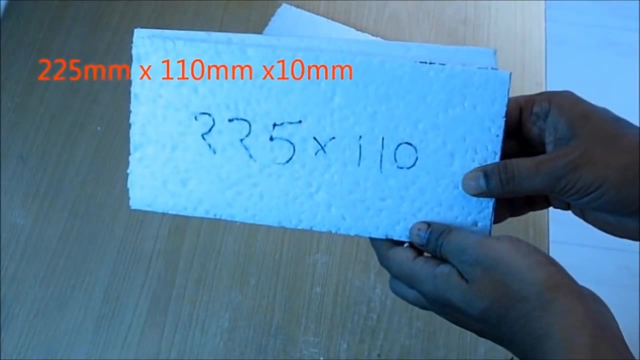 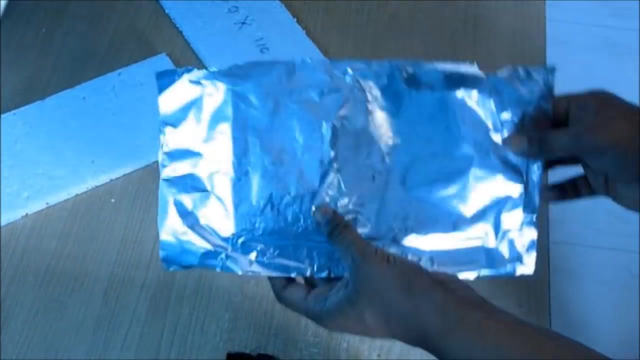 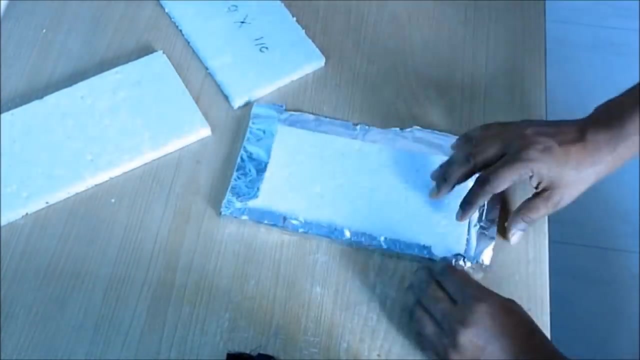 top of this thermocol. this will be the base of the cooker. cut four thermocol pieces, two of same size. each one is one centimeter thick. the sizes are shown on the screen. now put glue on the thermocol and stick aluminum foil used in kitchen. fold the other side and stick it with a tape. remember the glazy part should be. 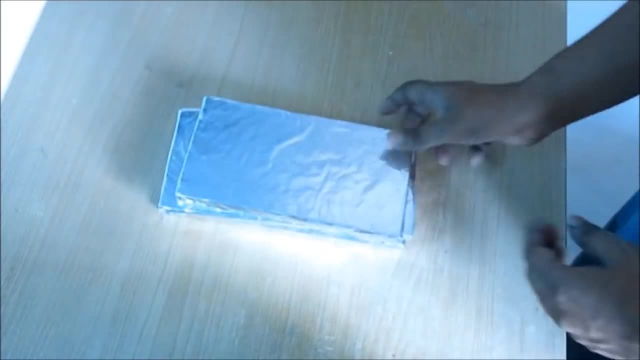 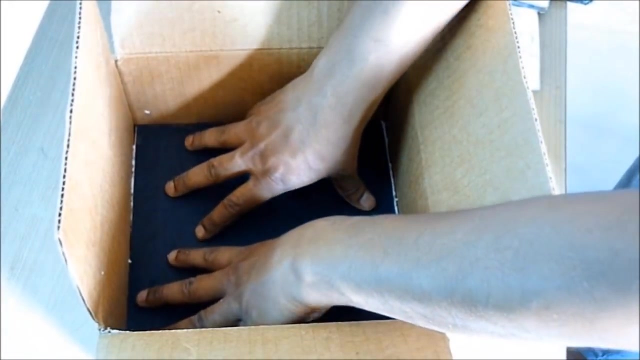 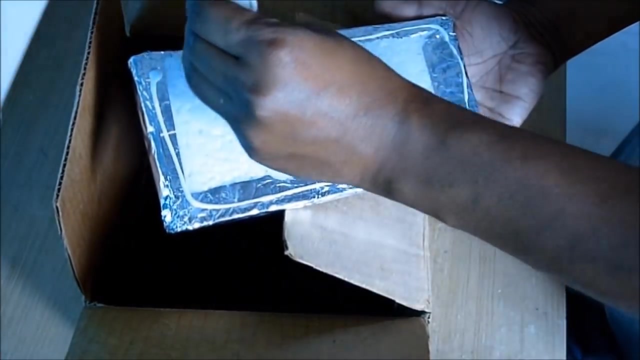 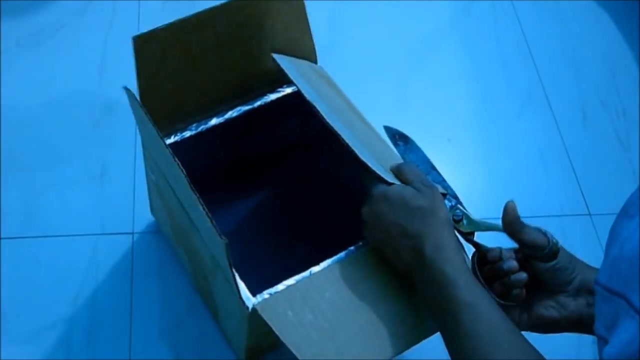 outside there's, I make total four walls. now put glue on the base of the box and put this thermocol concentrate. then glue all the four thermocol walls and all four sides like this. once done, cut all the top cover, keeping one about two centimeters side like this: ok, now cut all the top cover, keeping one about two centimeters. 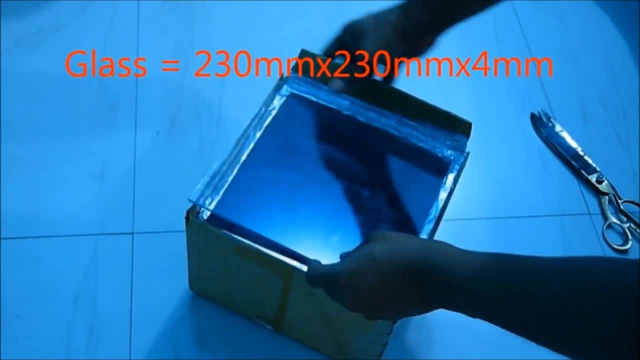 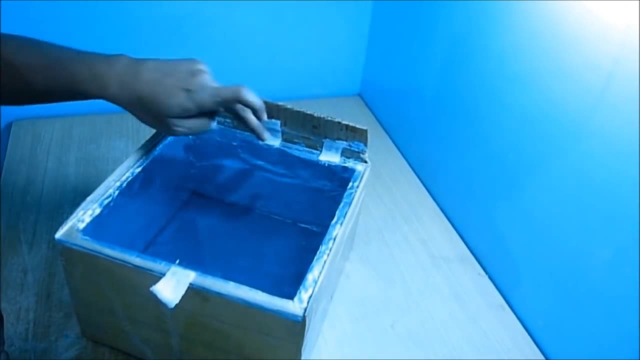 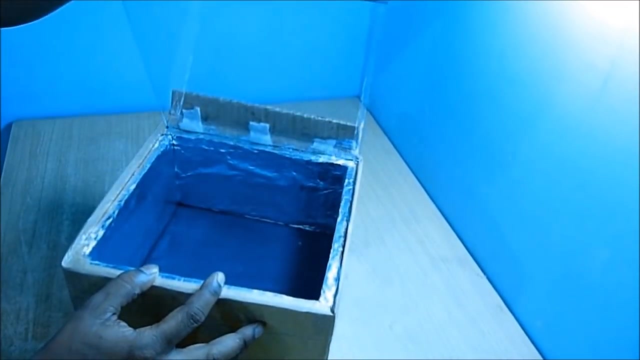 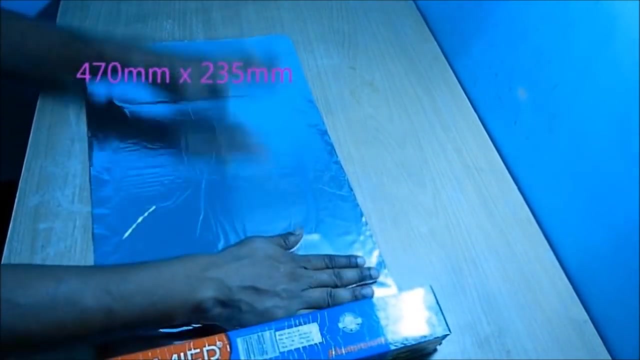 long i had a glass. i have to fix it on top of it. for that i have used this kind of cotton tape and hard glue. i stick this on top of it and i use a handle also for this to open the glass like that. now we have to make a reflector. the size is shown on the screen, put a aluminum foil on top of it. 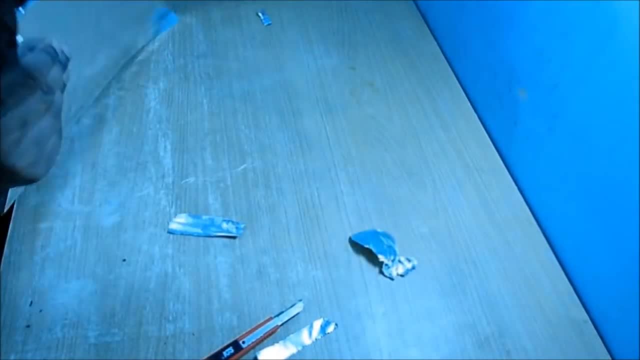 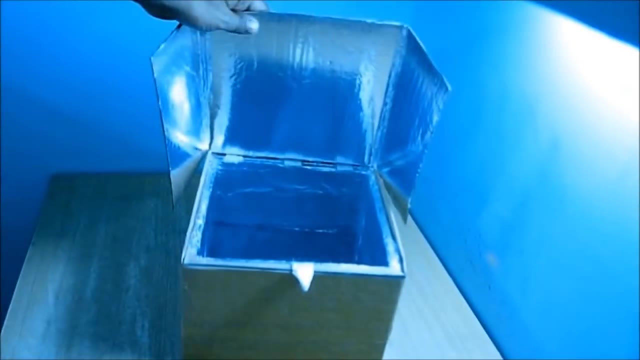 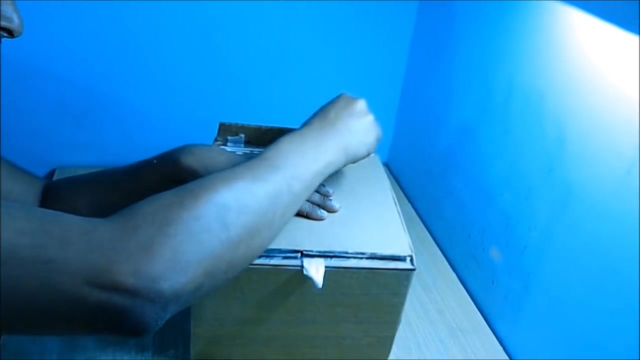 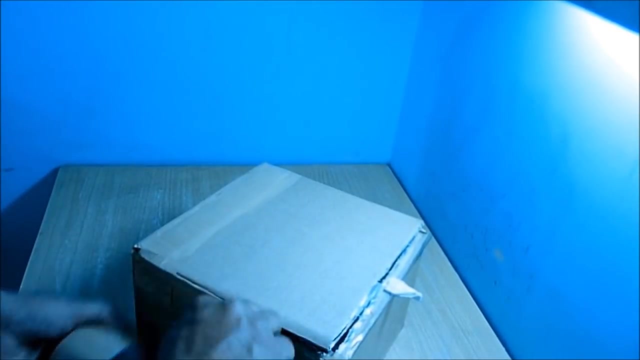 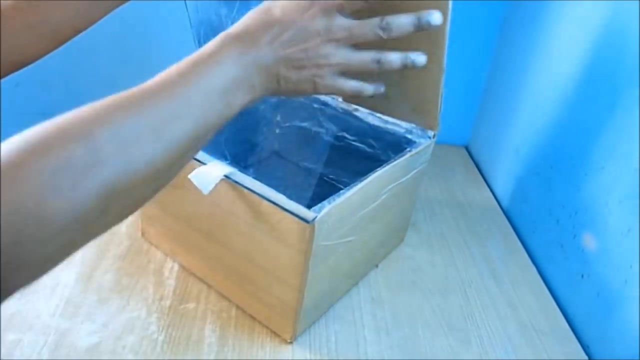 glue it and cut the extra out. this is the reflector. fold it. now we have to stick it on top of this box. put a glue and stick the extra out- cardboard coming out from that. using glue and brown tape like this. once dried up, you make some holes on top and use a wire to set the angle. so 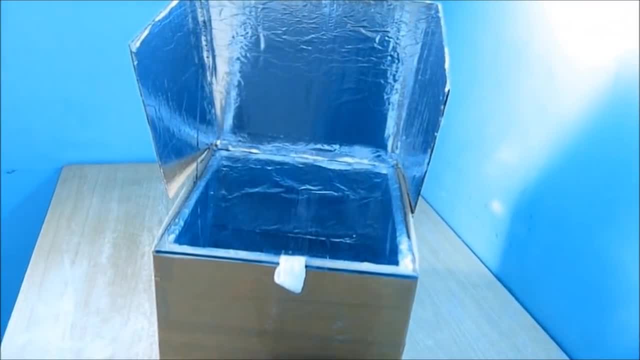 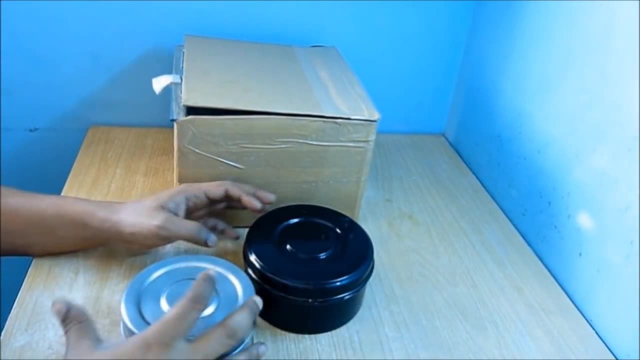 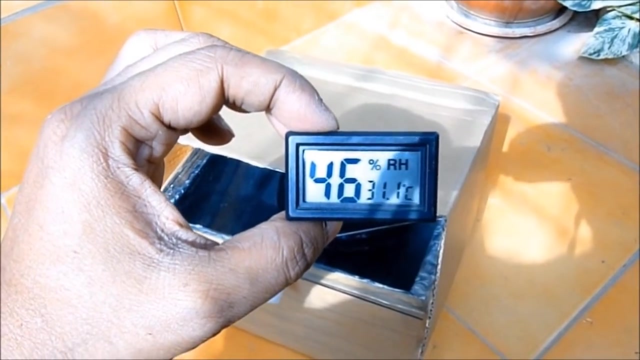 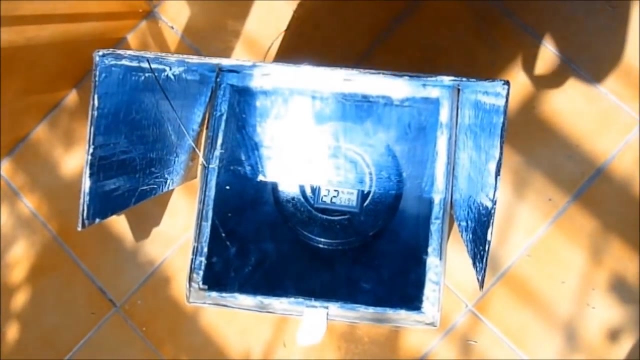 that the sunlight gets reflected and directed inside the two kind of tiffin box or cooking utensils you can use. one is black, one is white. let's try something today: very hot, 31 degrees centigrade outside. i kept this for around five minutes outside and the temperature raised to 51 degree centigrade. Today, cloudy, but let's try to.